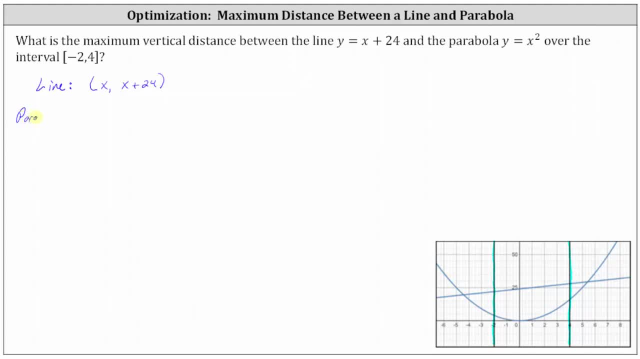 and any point on the parabola is going to have an ordered pair of x comma y, where y is x squared. And now if we take a look at the graph, well low, we are only concerned about the closed interval from x equals negative 2 to x equals positive 4.. Notice, over this closed. 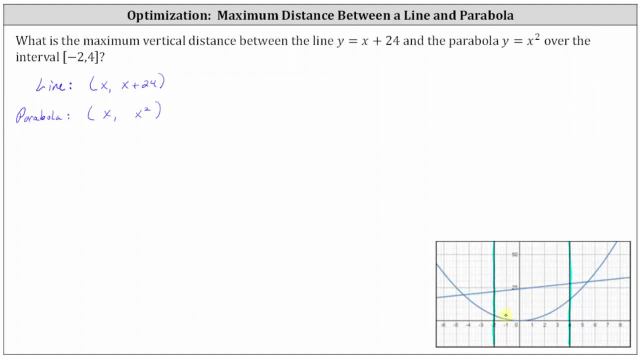 interval. the line is always on top and the parabola is always on the bottom And therefore any vertical distance, as long as the x coordinate is the same, is going to be the y equals 4. y-coordinate of the line minus the y-coordinate of the parabola. So, again going back up to our 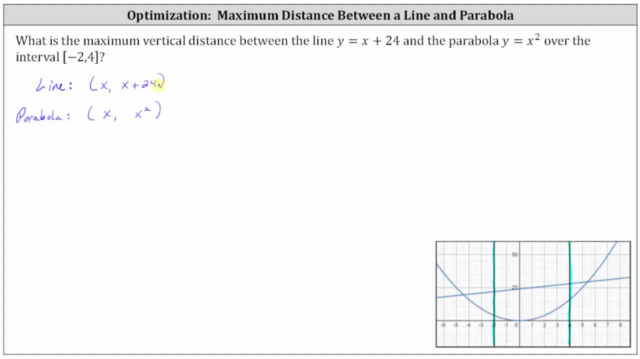 ordered pairs where, if the line contains the point x comma x plus 24, and the parabola contains the point x comma x squared, because the x-coordinates are the same, the vertical distance, which we'll call v, will always be the quantity x plus 24. 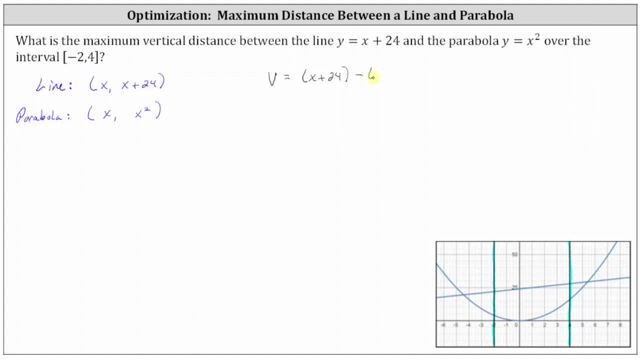 minus x squared, as long as the line is on top and the parabola is on the bottom, which is our case, over the closed interval from negative 2 to positive 4.. Let's go ahead and rewrite this as negative x squared plus x plus 24.. 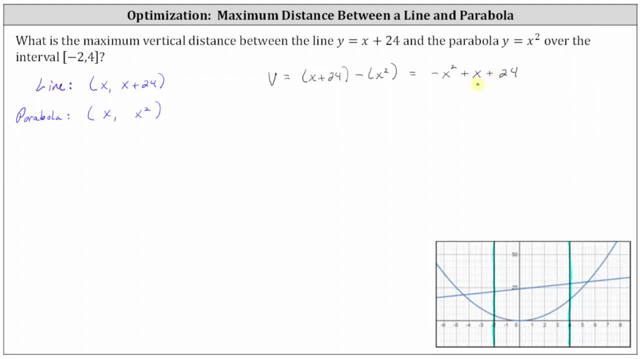 And we're trying to maximize the vertical distance. We should be able to recognize v is a quadratic function, but the graph is a parabola that opens down because the leading coefficient is negative 1. And therefore the maximum will occur at the vertex. But we will use calculus techniques. 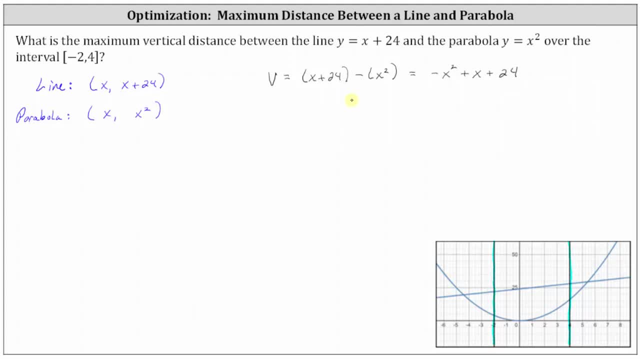 to maximize the vertical distance by next determining the critical numbers, which is where the first derivative is equal to 0 or undefined. v prime is equal to the derivative of negative x squared plus x plus 24 with respect to x, which is negative, 2x plus 1.. 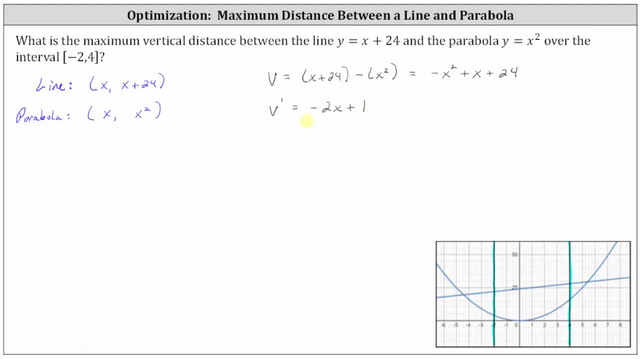 There are no values of x where the first derivative is undefined, and therefore we determine the critical number by setting the derivative equal to 0 and solving For the next step. we subtract 1 on both sides and then divide both sides by negative 2.. Simplifying, we have: x equals 1 half. 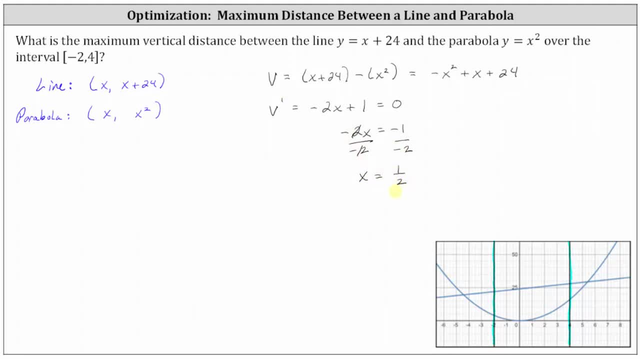 This should be the location where the vertical distance is maximized, and we can verify this a couple ways. Again, we know we have a parabola that opens down and therefore this will be the x-coordinate of the vertex. But if we're using calculus techniques, 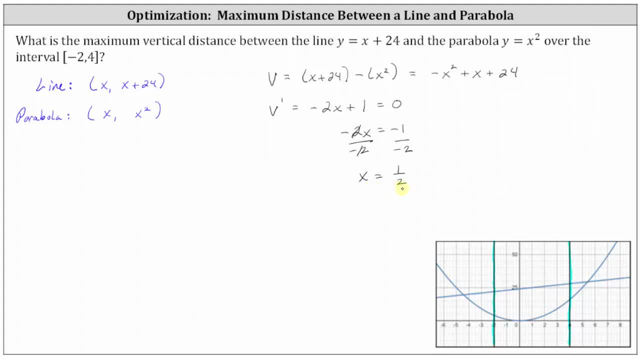 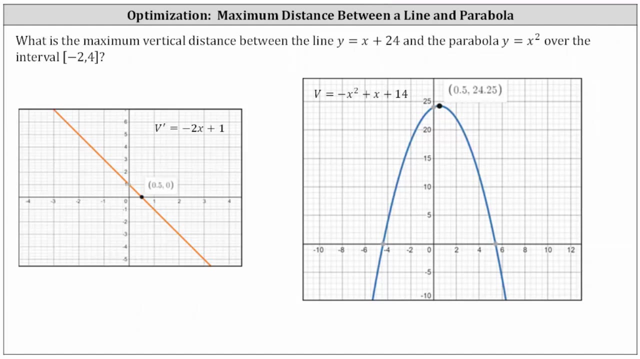 we need to verify that x equals 1 half. The function v changes from increasing to decreasing and therefore has a relative maximum at x equals 1 half. For this lesson, let's verify this graphically. So on the left I have the graph of v prime. Notice how the derivative is equal to 0 at x. 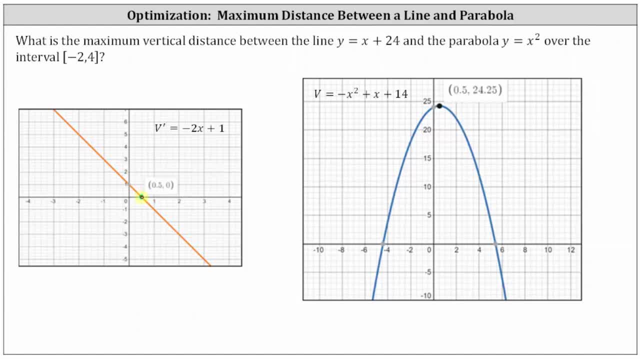 equals 1 half or 0.5.. Also notice how, at x equals 1 half, the derivative changes from positive to negative, which indicates that the derivative is equal to 0 at x equals 1 half. So on the left I have the graph of v prime. Notice how the derivative is equal to 0 at x equals 1 half or 0.5.. 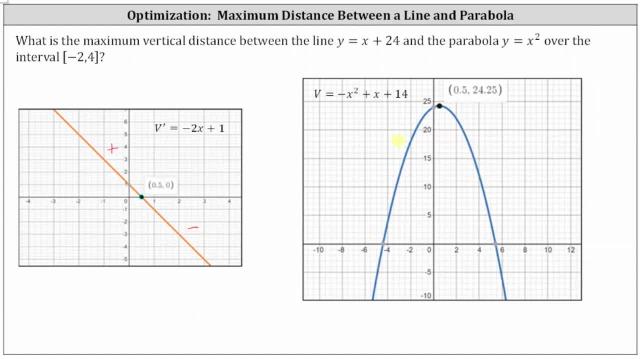 The vertical distance function v changes from increasing to decreasing at x equals 1 half. verifying: we do have a relative maximum or, in this case, an absolute maximum at x equals 1 half. But again, this question is asking for the maximum vertical distance, which is the value of v. 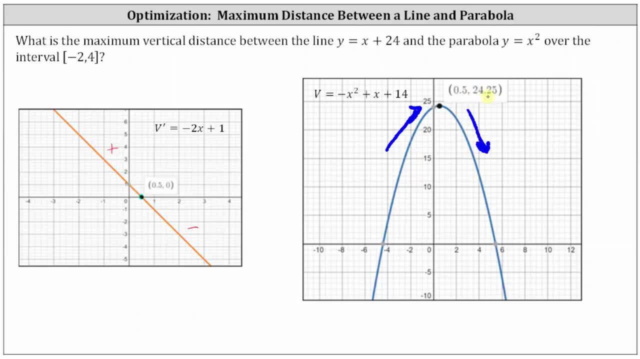 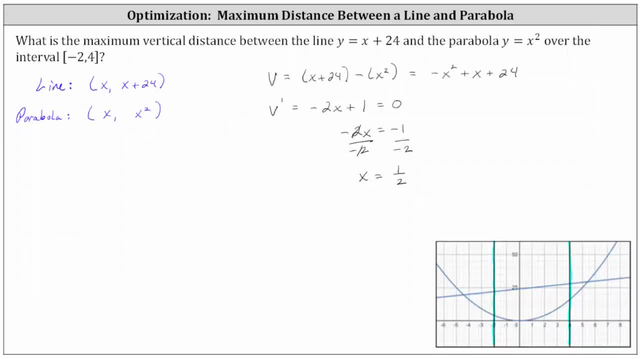 which we can see here is 24.25.. So 24.25 is the maximum vertical distance which occurs at x equals 1 half. So, going back to our first slide, we now know x equals 1 half is the location of the maximum vertical distance. And let's just verify the vertical distance that we saw. 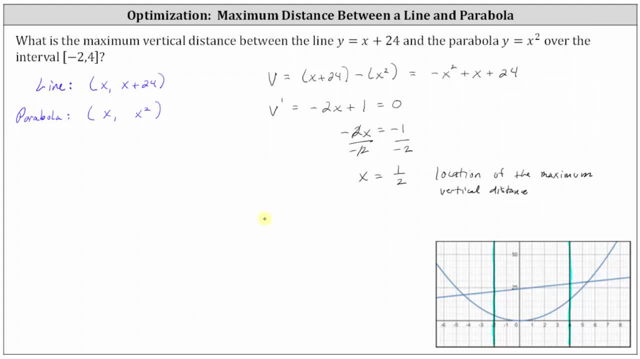 on the graph by determining v of 1 half. v of 1 half is equal to the opposite of the square of 1 half. Notice: the negative is not being squared and is not inside the parentheses. Then we have plus 1 half. 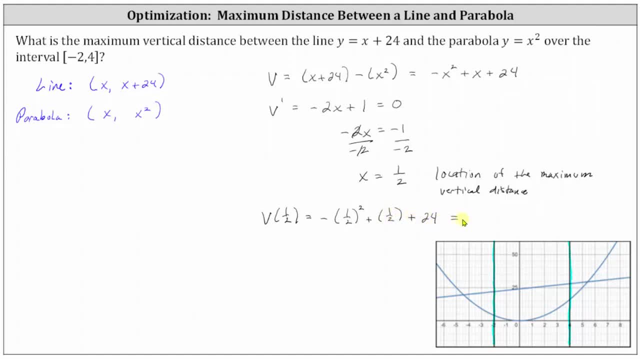 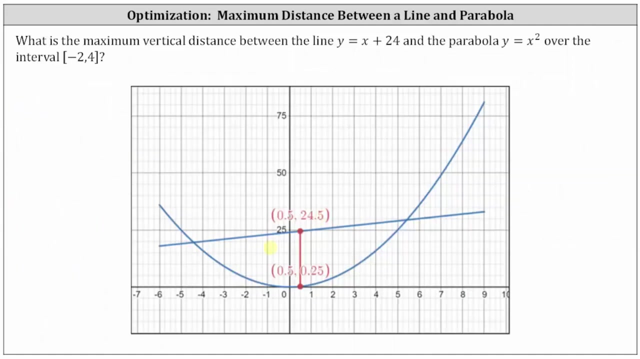 Plus 24.. Which does give us 24.25.. So, as a complete sentence, the maximum vertical distance between the line and the parabola over the closed interval from negative 2 to positive 4 is 24.25 units. And before we go, let's take a look at this vertical distance. Notice when x equals 1 half or 0.5,. 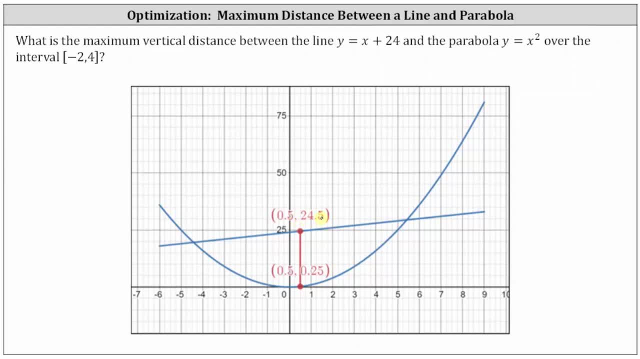 the point on the line is 0.5 comma 24.5.. And the corresponding point on the parabola is 0.5 comma 0.25.. And notice: 24.5 minus 0.25 is 24.25.. And 24.25 is the maximum vertical distance.